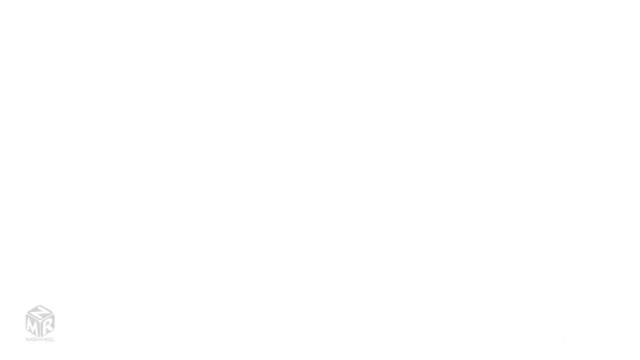 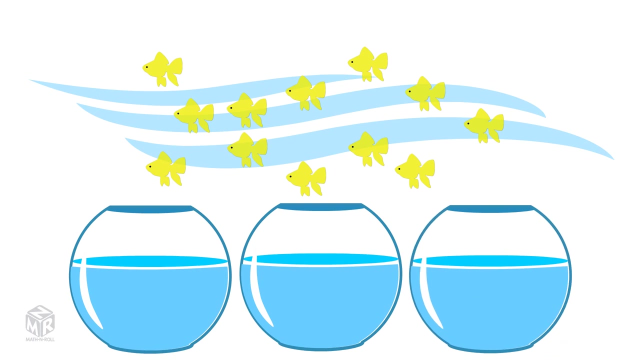 What is division? Imagine you have 12 goldfish. You want to move your fish equally into three fish bowls. How many fish will you have in one tank? Let's add the fish, one at a time, into each fish bowl. Now we have one fish in each tank. 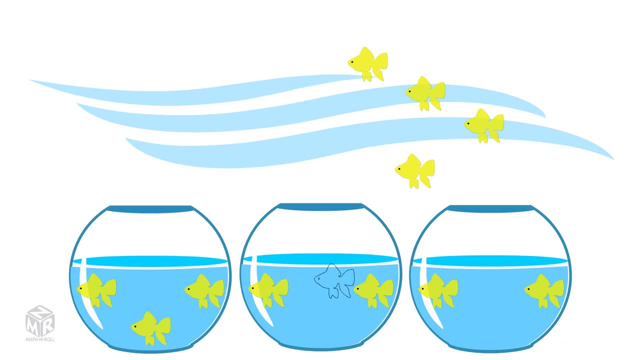 Two fish in each tank. Three fish in each tank, Four fish in each tank. Can you guess what we just did? We just used division. We divided our 12 fish into three groups. Now we have four fish in each group. Division is breaking up a number. 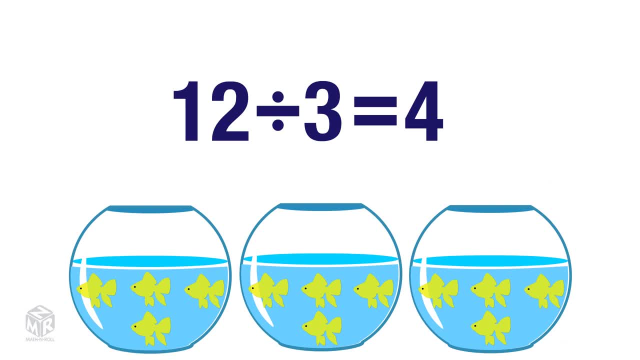 into equal parts or groups. Each part of a division equation has a name. The dividend is the divisor and the quotient. The dividend is the number that we are dividing in the division problem. The divisor is the number that you are dividing by The quotient is the answer. 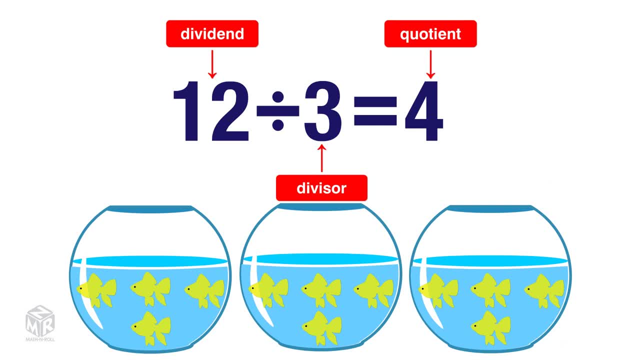 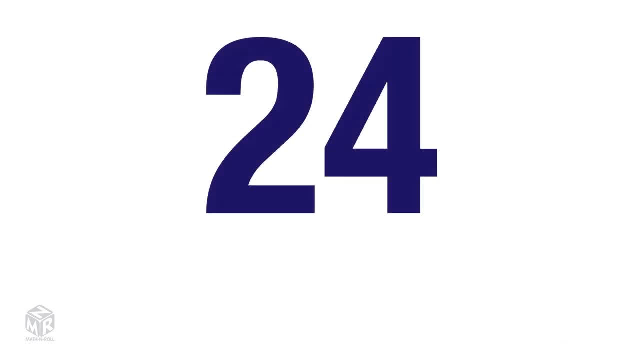 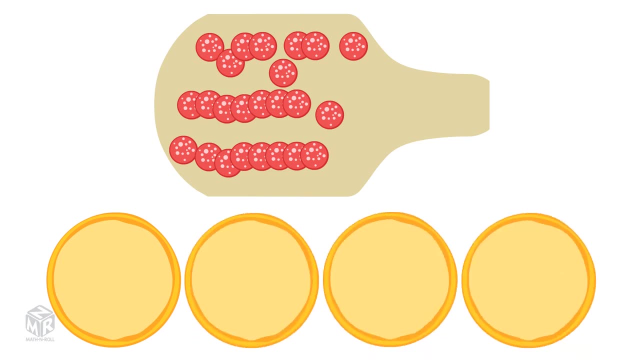 In this problem: 12 is the dividend, 3 is the divisor and 4 is the quotient. Let's try another example. We have 24 pieces of pepperoni. We want to put the pieces of pepperoni equally onto four different pizzas. How many pieces of pepperoni will be on? 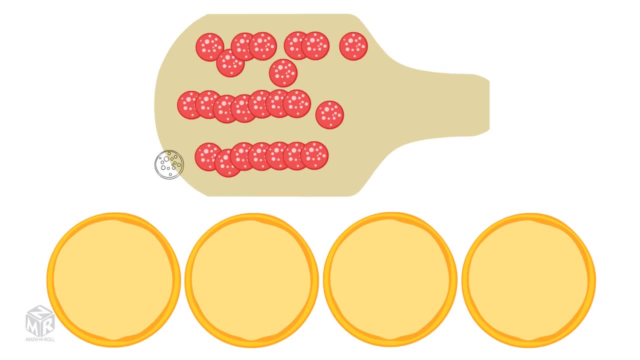 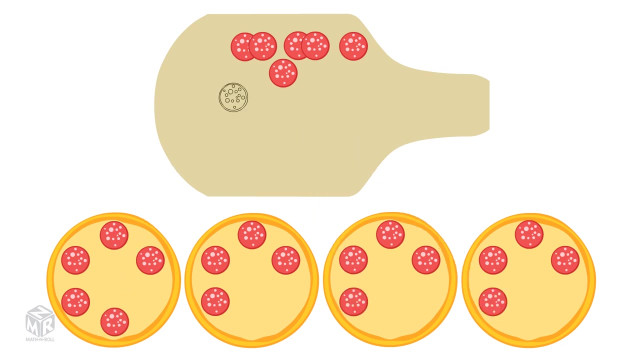 each pizza. Let's start sorting our pepperoni. We have one piece of pepperoni on each pizza, Two pieces, three pieces and so on. Each of our pizzas has six pieces of pepperoni. We want to put the pieces of pepperoni equally onto four different pizzas. How many pieces of pepperoni will be on each pizza? 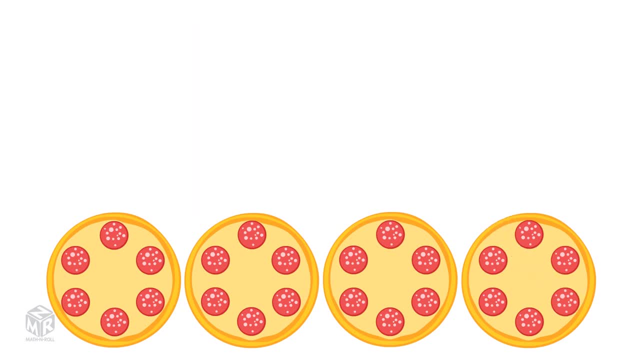 Our pizza has 6 pieces of pepperoni. We had 24 pieces of pepperoni and we divided them into 4 equal groups. Each group had 6 pepperonis. So now we have our division equation: 24 divided by 4 equals 6.. 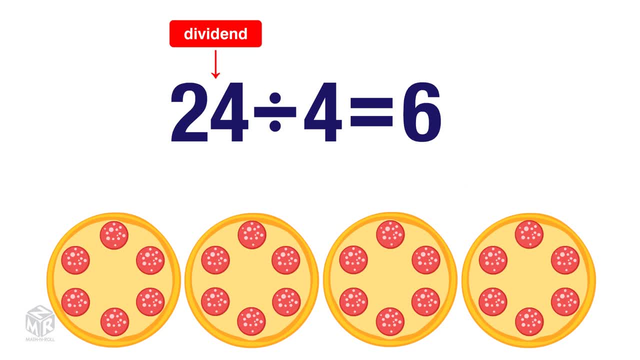 24 is our dividend or the number that is being divided, 4 is our divisor, or the number that we are dividing by, And 6 is our quotient or the answer. If you thought this video was helpful, please leave a like.